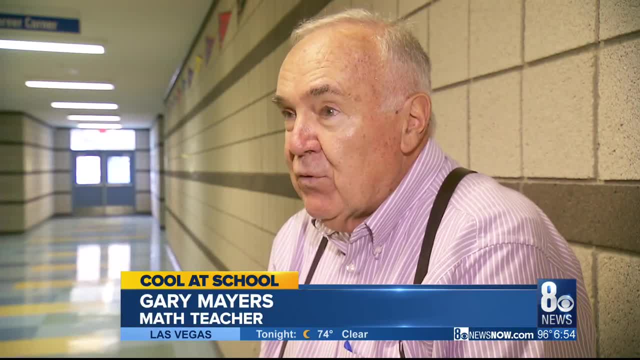 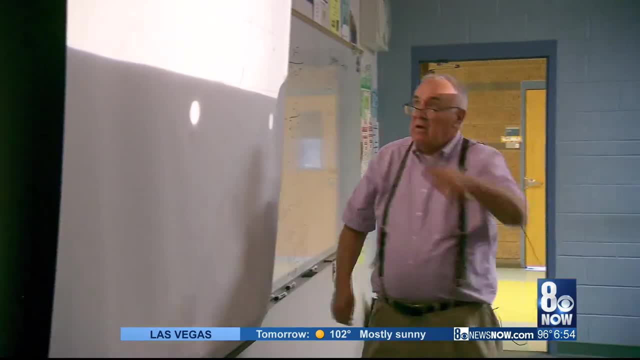 I bring a lot of humor into it. I love corny jokes. My first day in my other class I went like this: Gee, I'm a tree. Sometimes a little geometry or pre-calc humor is just what a kid needs to feel at ease and focus. 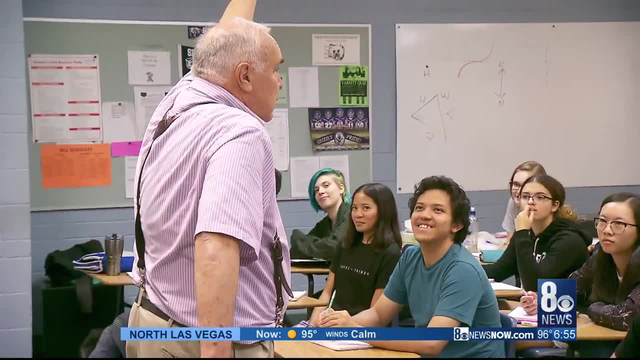 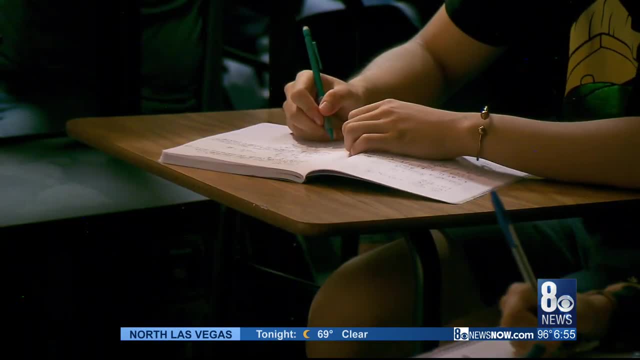 They love him, They love his humor. Is that right? Is the line going up? One former student, Cody Clark, now a teacher himself at Spring Valley, uses what he learned as Mr Mayer's student in his own class. I'm not afraid to be myself in front of my students. 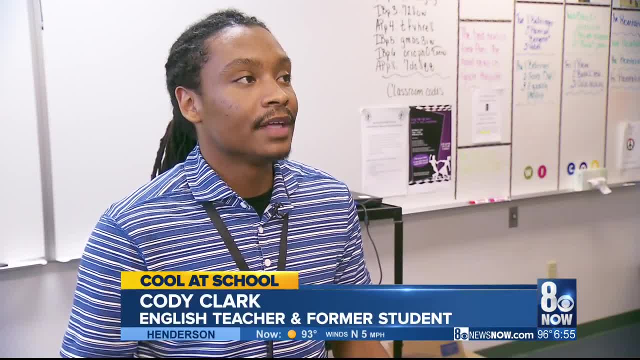 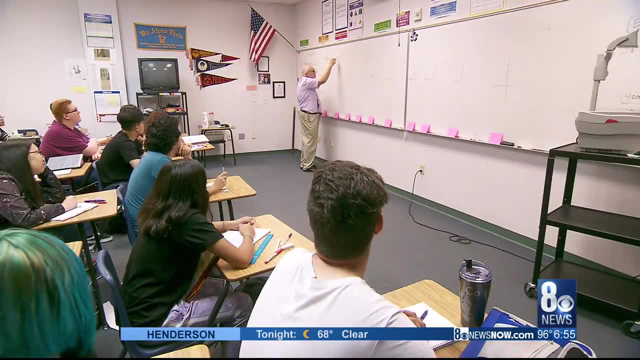 I'm not afraid to be a person, be personable for the students, And I think that had a lot to do with him: Five and a half decades of experience and a proven track record of high achievement from his students. Maybe this is a more challenging lesson than I thought. 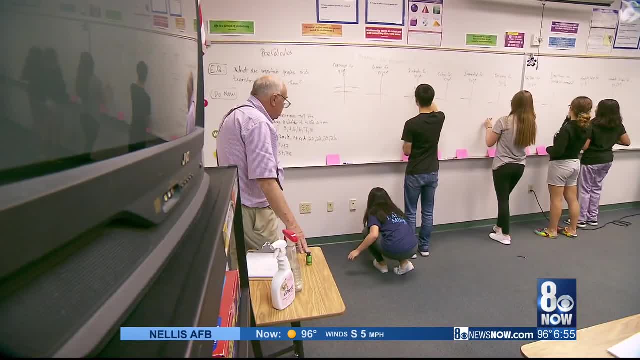 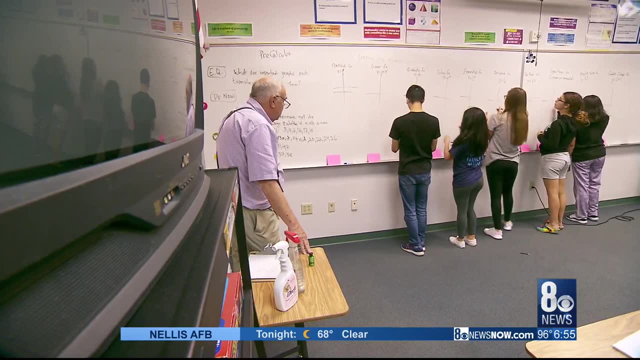 Well, I have good news for you. At least one of them is right. Some possible reasons for his success: Success: Selflessness. He's always available to help them. He'll do whatever he can to help a kid. If I didn't understand, I could go after school and like, even when he's eating lunch by himself. 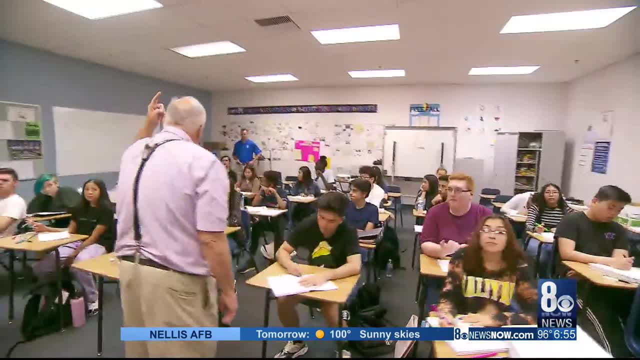 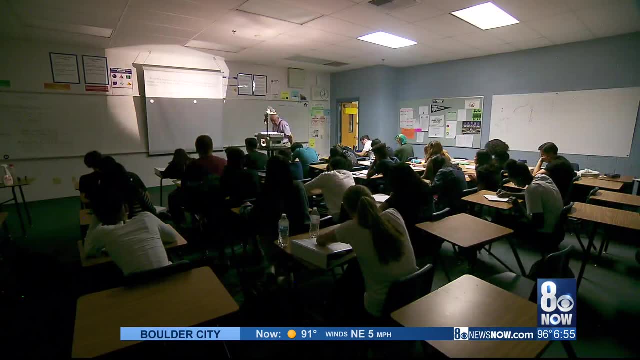 he'll like give up his time to like help me understand Also the way he feels about teaching and his students. He just loves what he does, His love of students, The fact that I get an awful lot of enjoyment about taking somebody who didn't see something. 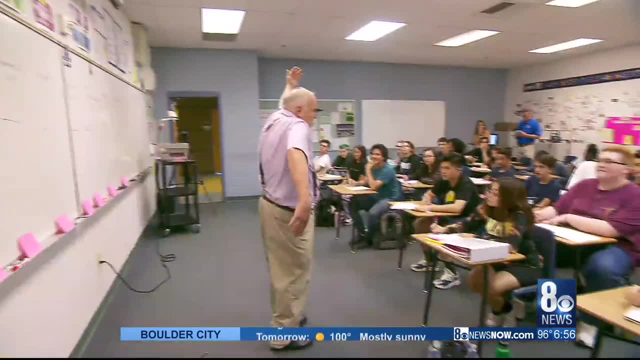 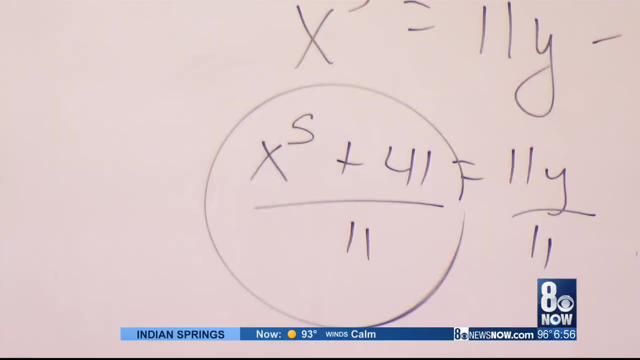 and getting that aha moment to understand something. Is it going in the right direction? Because to me it's backwards. There are some people that are just born genuine teachers, and he's one of them. His advice for the new teacher may be fresh out of college, a bit green. 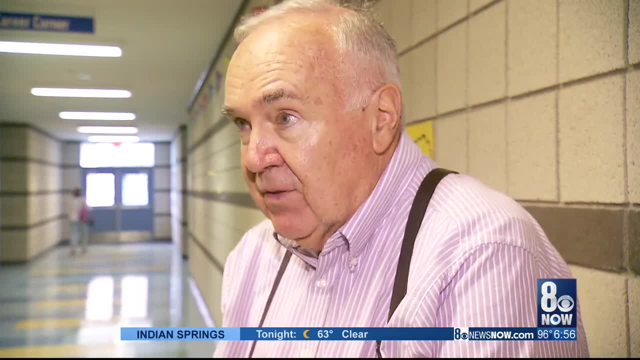 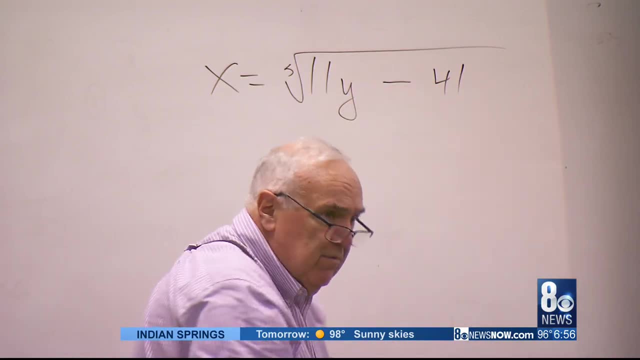 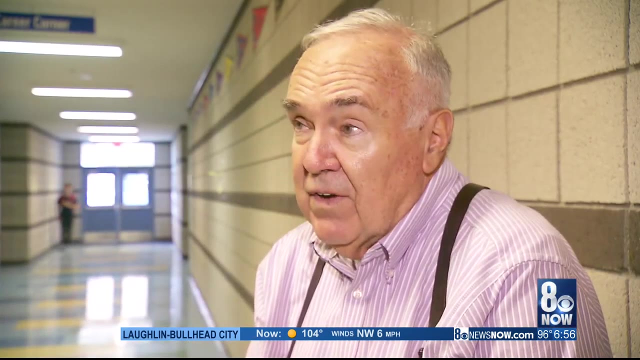 Have variety. Don't do the same thing. Do different things. Sit in a room of experienced teachers as much as you can. Go to different teachers. Gary Mayers was rightly recognized as the 2011 Presidential Award winner for math. Well, I was one of the oldest teachers ever to get that. I got it at age 65.. 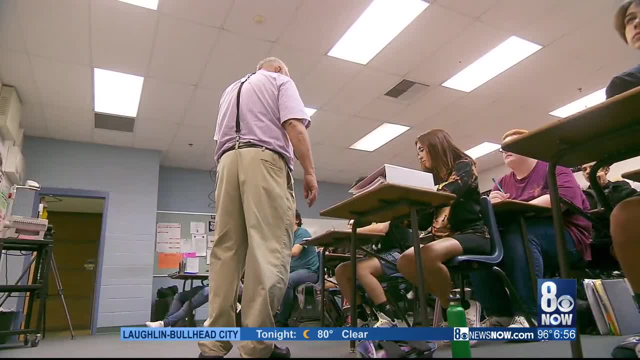 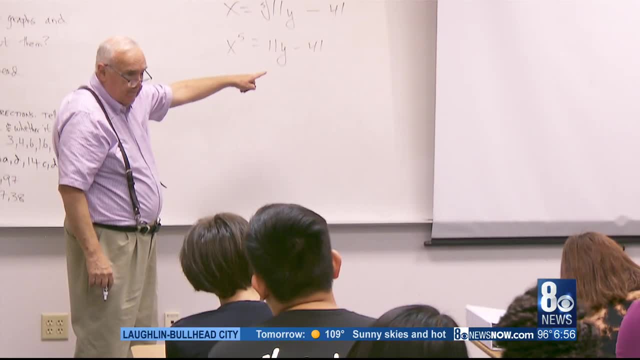 And to me it was a reminder: I was one of the oldest teachers ever to get that award. I was one of the oldest teachers ever to get that award. Fifty-four years of helping kids understand a notoriously difficult subject, making them smile and lifting them up with his positive energy.